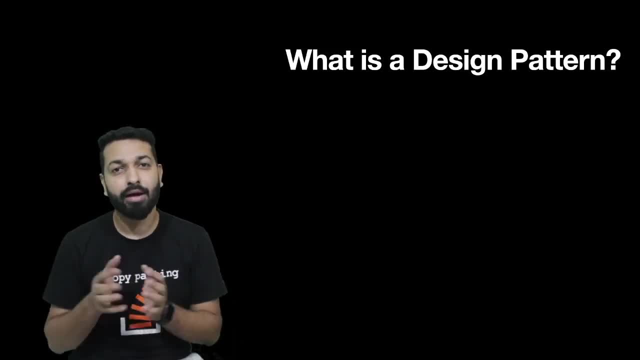 MVVM, Viper, MVC, MVP. And when I ask about architecture, they tell about singleton observer. So these are two different things. Don't put one in place of another. Architecture is for the entire application, That how your application is built, the overall. 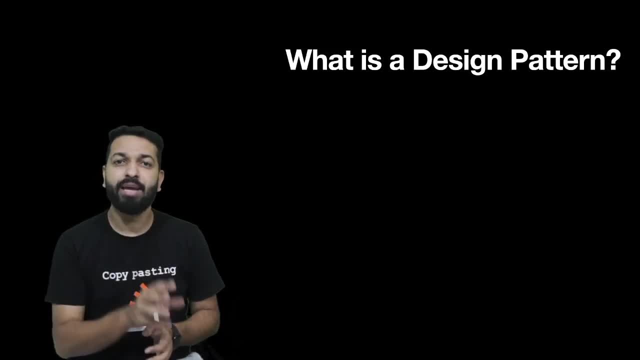 structure of the application, the overall architecture of the application, While design pattern are for the smaller modules. You can treat it as design patterns eventually contribute to your architecture. So, for example, you can have singleton for some specific module, you can have observer pattern for some other module, you can have facade for some other module. 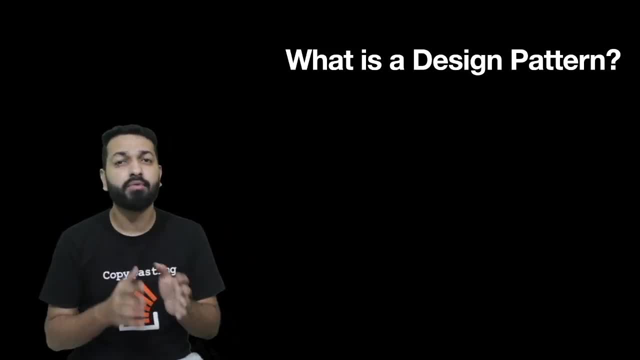 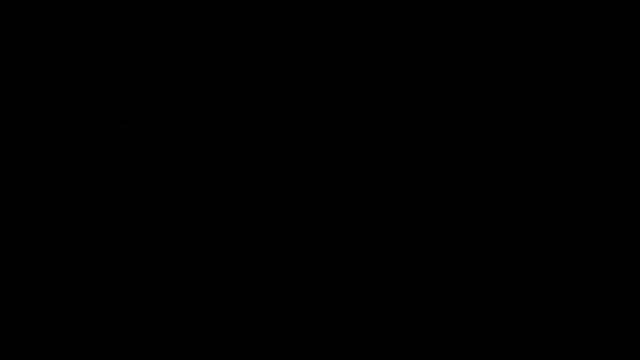 which, in totality, will make the MVVM, Viper, MVC, MVP, whatever you are dealing with. So architecture is for entire application And design patterns are for specific modules. Don't confuse them. And the second point is that: why should we use design patterns? 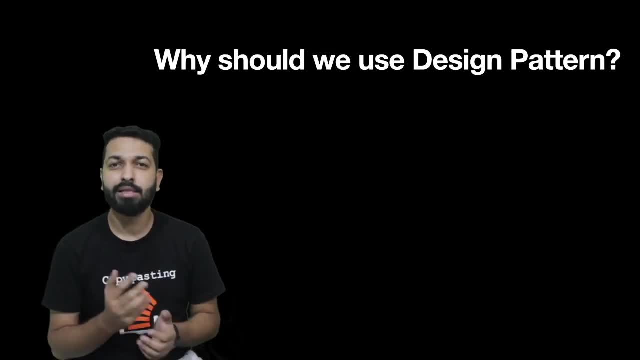 So design patterns makes your code more manageable, more scalable, easily testable. It breaks into the modules Many times. the issues that you encounter at a very later stage of development are identified right at the beginning of the development when you use design patterns. 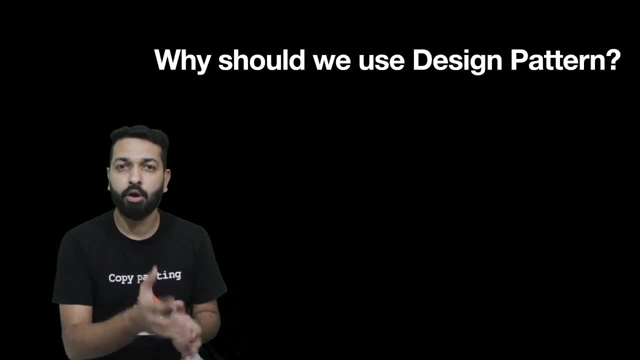 So these patterns have evolved over time, looking at those issues, the potential problems, those situations and considering everything. So there should be no doubt about why to use design patterns. It will make your life easy. Apart from this, design pattern also helps in communicating with other developers. 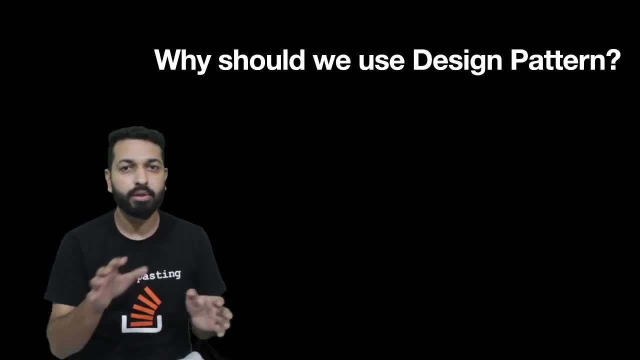 So let's say a new developer joined your team. Now he or she is not aware about the code. Obviously, new developer will deep dive into the code to understand that how it has been written. But if you say that you have used a particular design pattern for this particular module, and if he or she is aware about that design pattern, 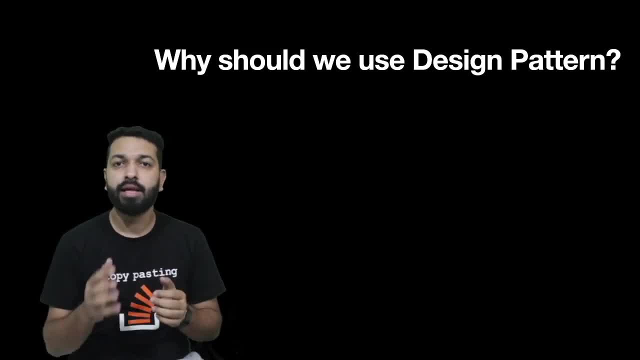 then it will get really easy for the new developer to get the hang of the code. So if you tell them that you have used singleton for this particular module and they already know that, okay, in singleton you will be having a shared instance and how it works, it will be really easy to pick up the code, to pick up the flow. 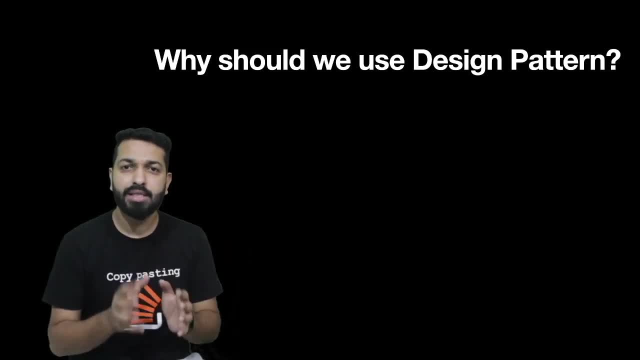 They won't invest their time in understanding the design pattern or the architecture. Instead, they will focus on understanding the business logic, and that is what you want. So if you use design pattern proper architectures, then it will eventually speed up the development process. 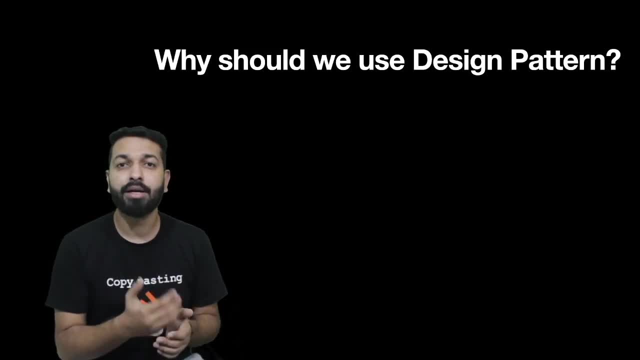 Of course, they are important for the interview, but I would say that they are even more important after the interview. So let's say that you have cleared the interview and you have been offered the role of the developer- Tech lead architect, senior software developer- and you have been asked to design a module. 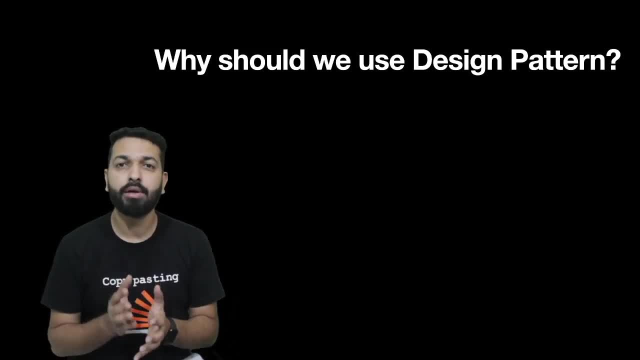 At that point in time, design patterns will come into the play. You will be evaluated on these skills of yours: How efficient system have you designed, What design patterns you have used, What architecture have you used And, eventually, how manageable, how scalable, your code is. 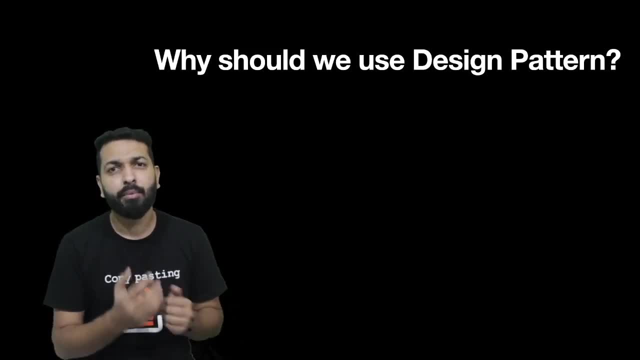 Your team will be following the pattern that you have decided. So, then, the importance becomes even more. Now let's see that. what are the different types of design patterns? This will be really quick. I won't deep dive into each of the design pattern. 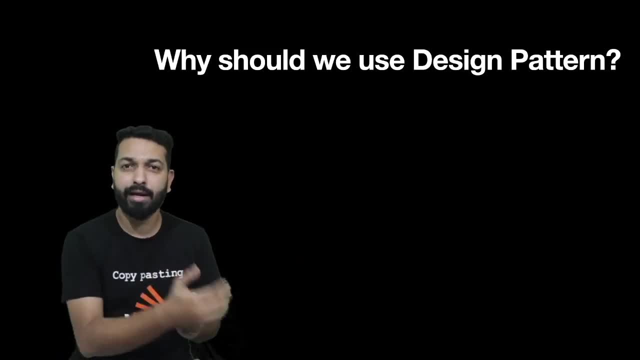 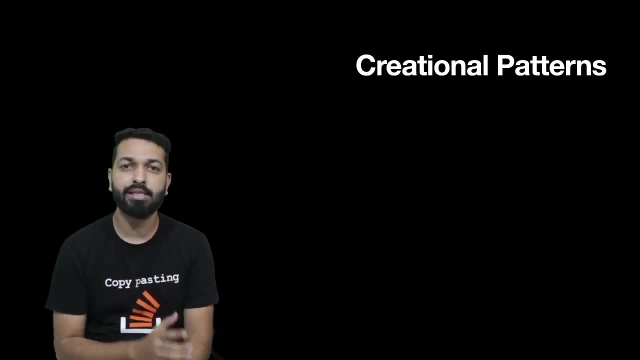 Instead, we will just see that. what are the different categories of design pattern, How are they categorized, And then we'll focus on factory design pattern. So the first category in which the design patterns are categorized is creational design patterns. Now, creational design patterns are those patterns which focus on creation of the object. 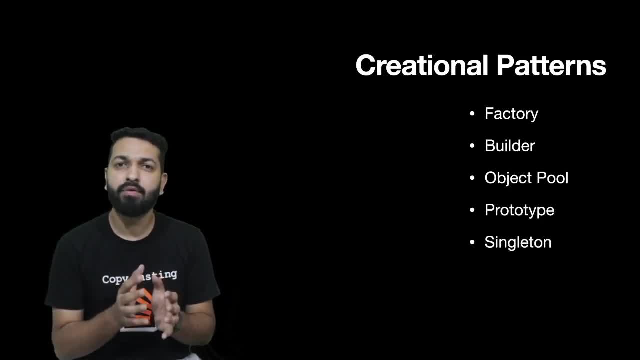 How an object is being instantiated. Their sole purpose, their entire focus is on the how part of the object creation. Now it might appear very lame and very easy to you that we can directly create an object by using the class name and then parentheses. 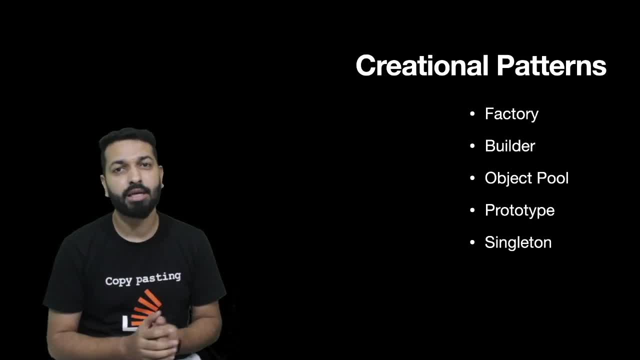 What is the need of a pattern? but you will understand this when we'll be discussing about the factory pattern in a minute. So these are a few of the creational design patterns. There are more than these five. Now let's see the next category, that is, structural patterns. 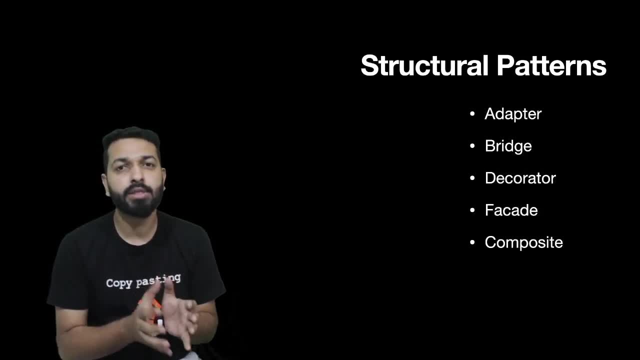 Structural patterns are those patterns which are concerned about the composition of a class or an entity in general. They are concerned about how a class should be composed so that it eventually contributes in building a larger structure. So, for example, facade- The literal meaning of word facade- is the front end of a structure. 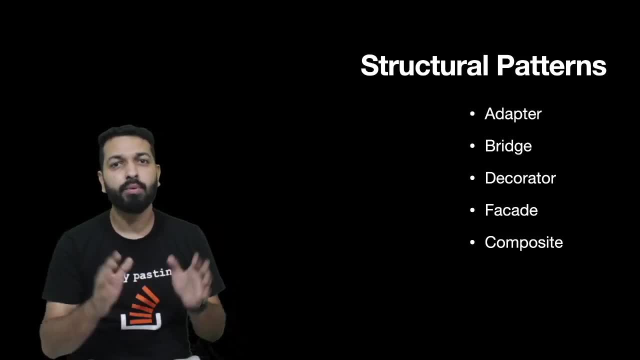 So, for example, facade Is the front of the building. So when you look at the front of the building you are only looking at the building from outside. You are not concerned about how plumbing work has been done. You are not worried about that, how power supply has been managed, how wiring has been done. 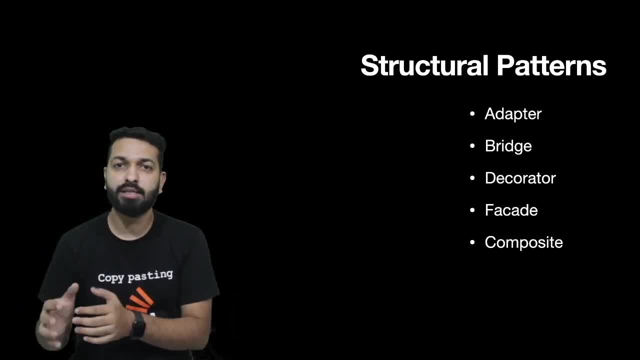 You are only seeing it from the front. So it focuses on the composition of classes that should eventually contribute in a larger structure. It concentrates on identifying the relationships between the entities. Let's not go too much into the details of structural design patterns And let's see our third category, that is, behavioral patterns. 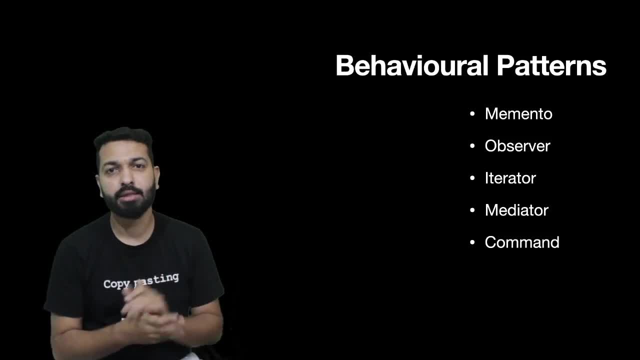 Behavioral patterns. Behavioral patterns concentrates on the interaction of the objects and their responsibility. It says that objects should be easily able to talk to each other, but at the same time they should be loosely coupled. So this was just about the classification of design patterns, and I'll try to cover each one of them. 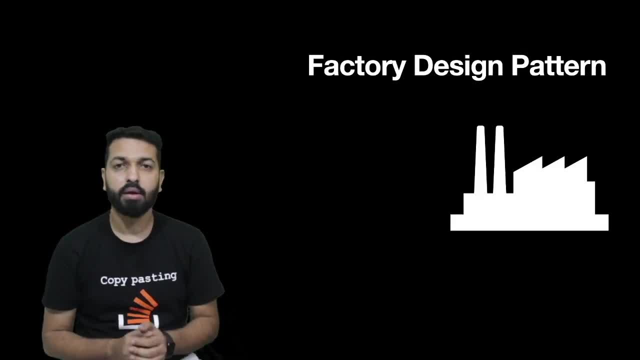 But for this video, let's focus on factory design pattern. Factory design pattern falls under the category of creational design patterns, And so it focuses on how to create the objects. So it says that there should be an interface, There should be a protocol. 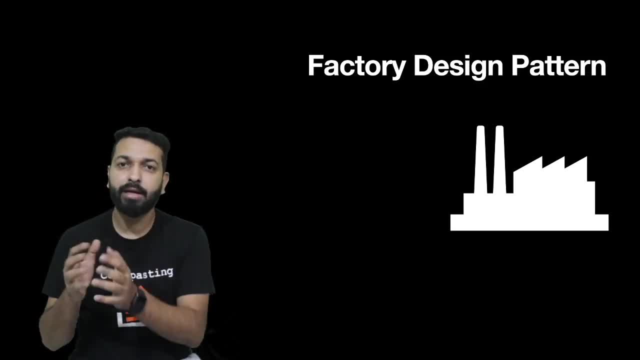 Which talks about The object creation, But the subclass or the entity that is confirming to that particular protocol should be responsible for identifying that what kind of object is to be created? And I understand that from the definition it is not at all clear. 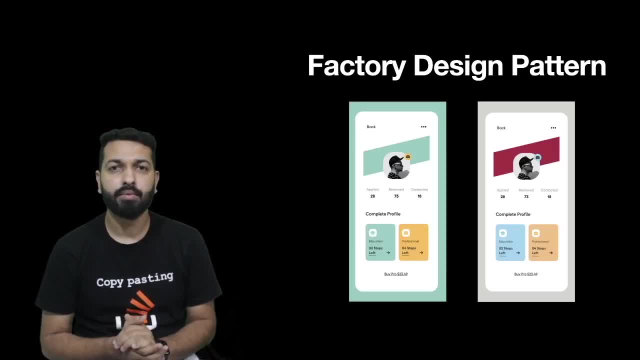 So let's take an example. So assume that in your application you need a profile view which should display the user's profile. Now the design of that profile view can change depending on certain factors. Product can come up with some weird requirement. 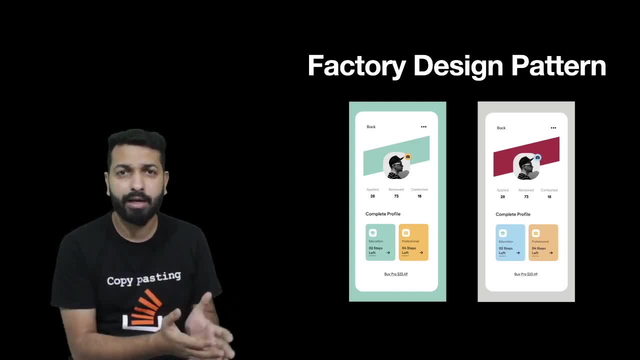 They guys can ask you to change the look and feel of the view depending on some weird criteria. It can be some festival, some event that let's say the Christmas is coming, So the profile should have the Christmas look and feel. or they can come up with some concept of privileged users, pro users. 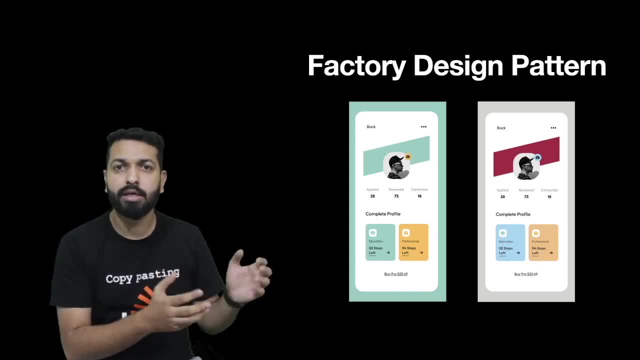 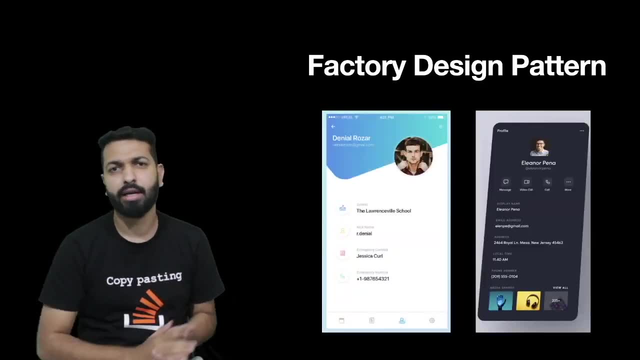 So there should be a simple layout, a simple view for the normal users and there should be a fancy view for the pro users, for the privileged users. Basically, different design depending on different situations, different criteria, and there can be 65,000 reasons for it. 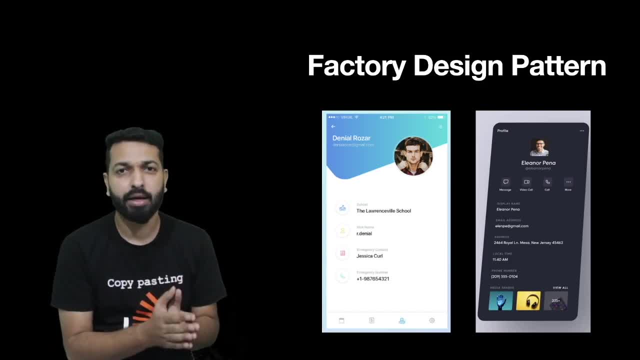 Now what factory pattern says here is that you should be having some kind of factory, Let's say profile view factory. You will just tell that factory that You want this particular kind of profile view and it will return it like that: Now you're not concerned about how that view is being created. 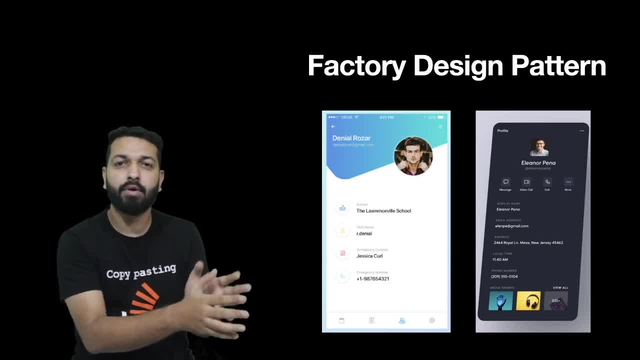 What is the underneath implementation of that? How is the object is being created? What is the complexity involved in the object creation and everything else? You are not aware about that. You are not concerned about that. You just ask the factory to give us the profile view and it returned to it. 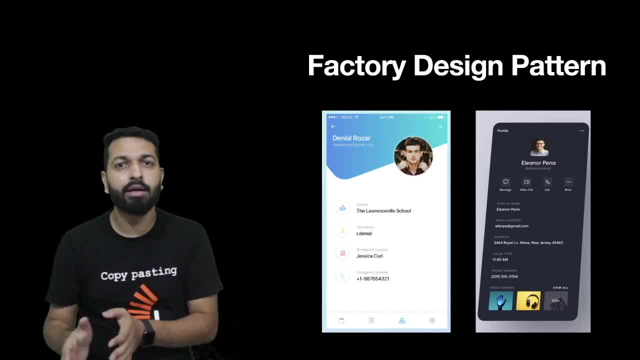 Now you are getting the profile view for the blue color theme, for the red color theme, for festival theme, for any festival, for any other event. You are getting the same profile view. Of course, the theme is different. That is your requirement. 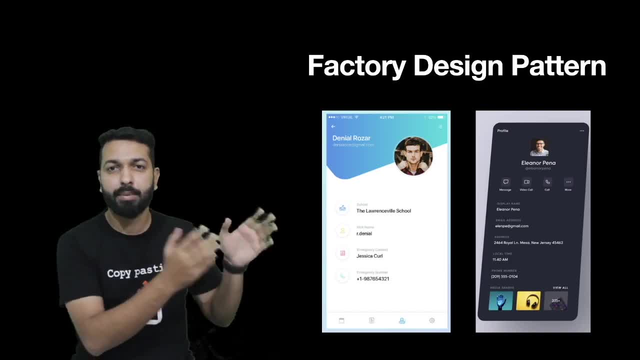 But the profile view is having the same components. It has a profile image, It has a label for the user name, It has some ratings of the user, It has some other preferences of the user. Those components are the same. The theme has changed or whatever changes that you wanted for that particular profile view have been made. 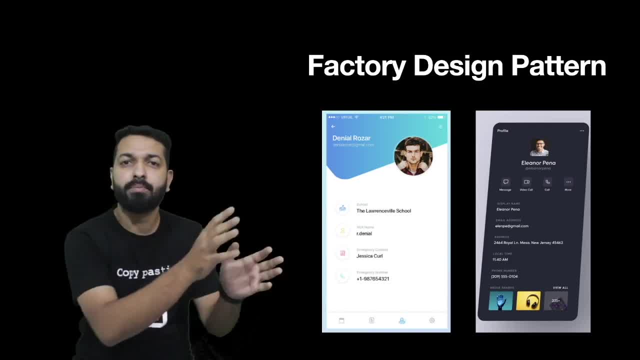 But you got the profile view object. Now this is what is being done by the profile view factory. Let's see that how it can be done. So what I mean to say is that let's see that how can you implement factory pattern. 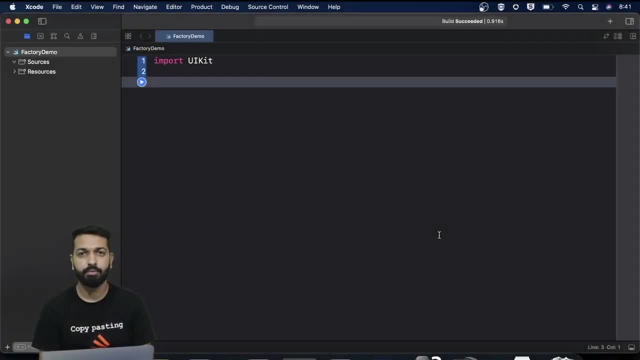 So let's start with what we want. We want to have a factory that should return us the profile view. So let's create one. So let's create our factory class, say class profile view factory, And then there should be a method which we will call and it will return us the profile view. 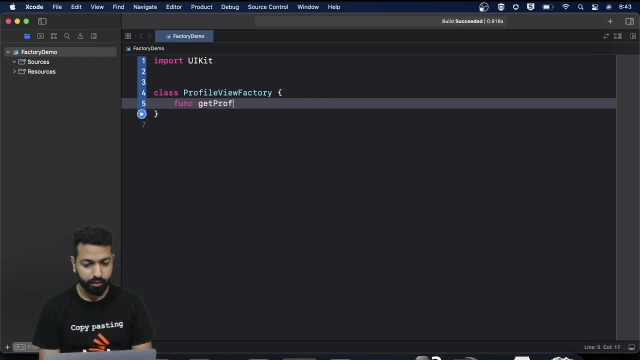 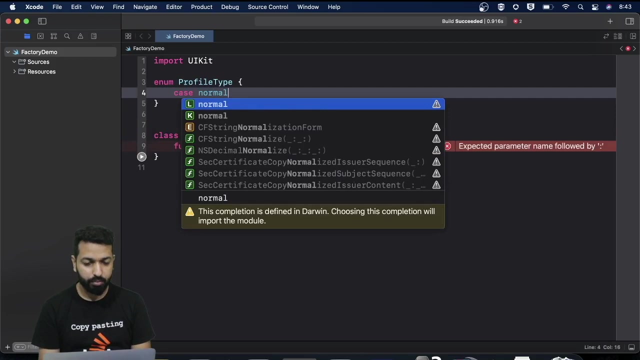 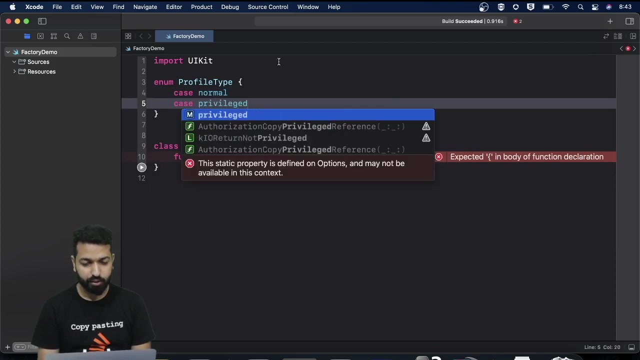 So let's create one, say func, get profile view. Now we want that we should be able to pass a type that we want a normal profile or we want a privileged profile, a superstar profile. So let's create, Let's create a type first, let's create an enum for that, say profile type. and for now let's just put two cases: say normal, and the second would be say privileged. 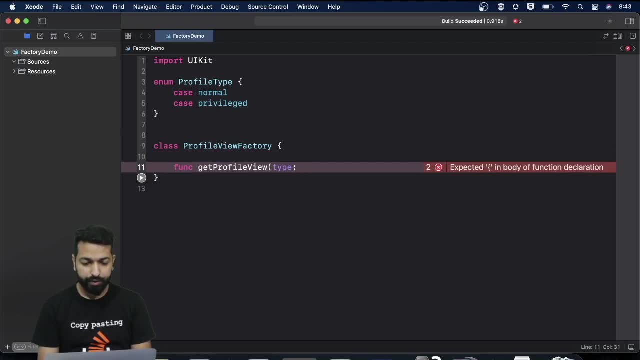 So this get profile view will get the type of the profile that will be profile type and based on this, it should return a profile view. So let's create a profile view first. But what will be a profile view? Will it be a class? 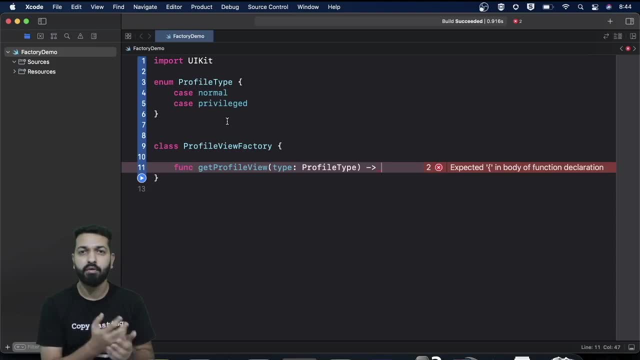 No, we actually don't want to return that concrete implementation. We want to return a protocol, an interface. So let's create one. So let's say protocol, say profile view, And then this profile view protocol should have those things which generally or which all of our profile views should have. 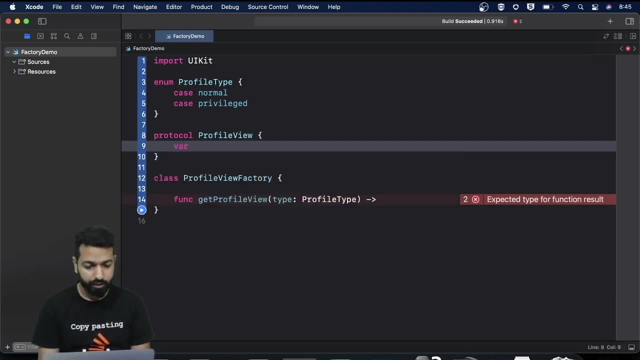 So it should have an image view for the profile image. So let's go for it Where: profile image view And this will be a UI image view. What else it can have? It can have a label for the username. So let's say where we use a name label. 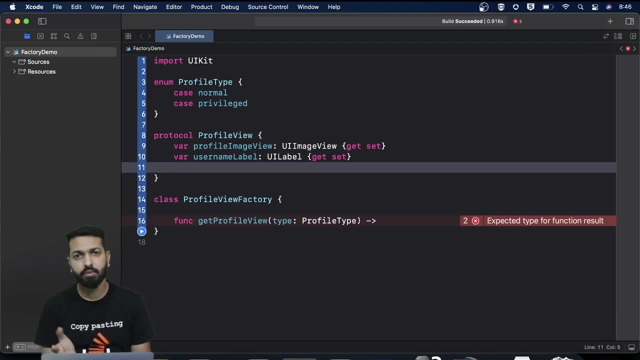 And it can have the points, the balance that user is having, if that is the use case. I mean, obviously these things will change depending on the use case, So let's just consider one. So I would say it Say: 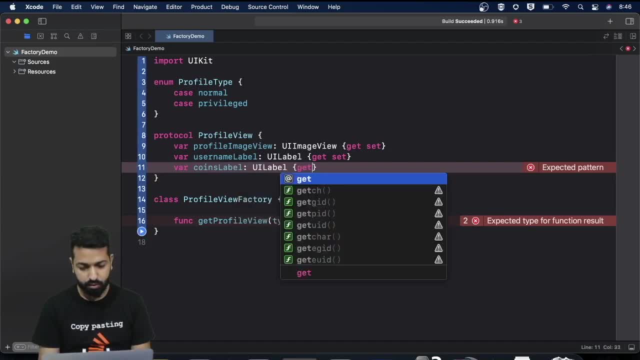 Points label. maybe this will be again a get or set. So this is a basic structure of what profile you will be having. There can be a lot more, but let's just consider only these three for now. Now we'll be returning this profile view from our get profile view method. 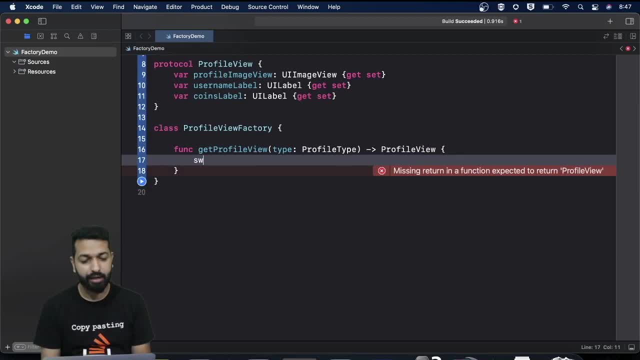 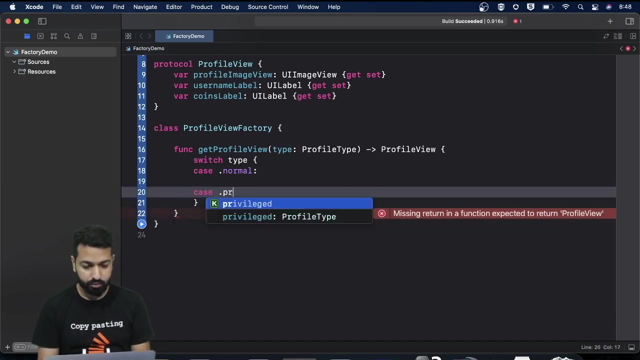 And inside that method we will have the checks for the profile type. So if I go for switch and switch on type, which will be either Normal or, it can be, say, privileged, in either of the cases we need to return a profile view. 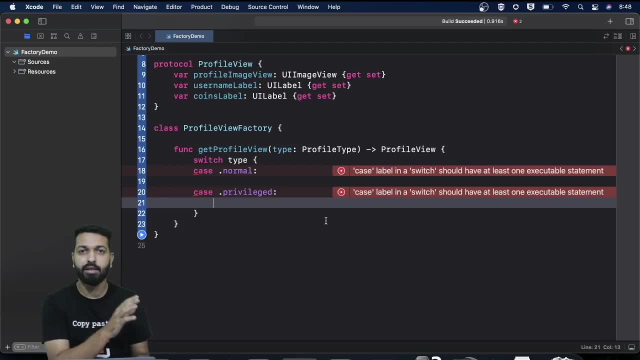 Now comes the point that actually, what will be returned? I mean, the protocol has been set, The interface is set, We have set the blueprint, We have set the guidelines. Now the concrete implementation. So for the concrete implementation, we can have the classes. 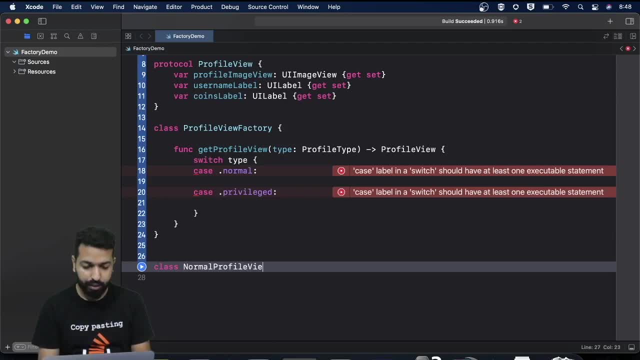 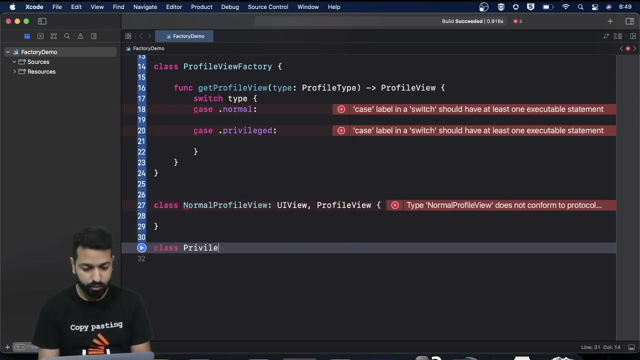 We can have the views for it. So let's say normal profile view, which will be a UI view, And it should Also consider to our profile view, say, and we can have one for our privileged users, So say class privileged profile view. 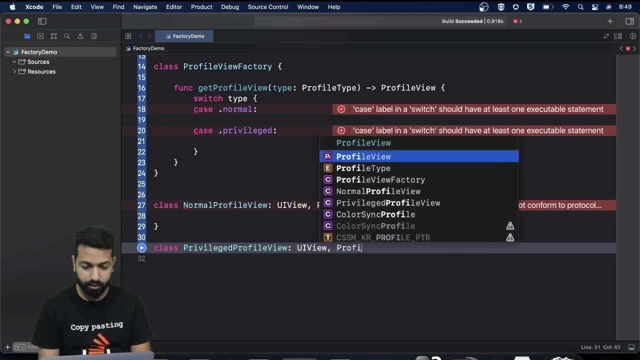 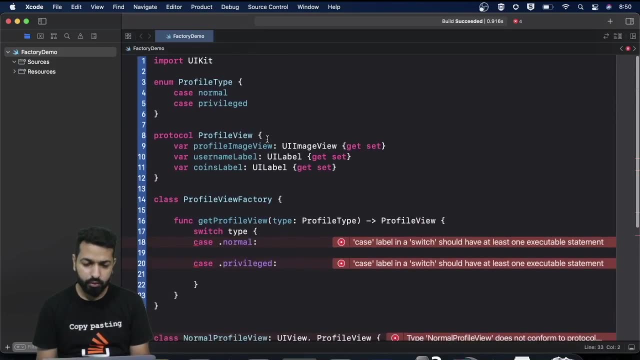 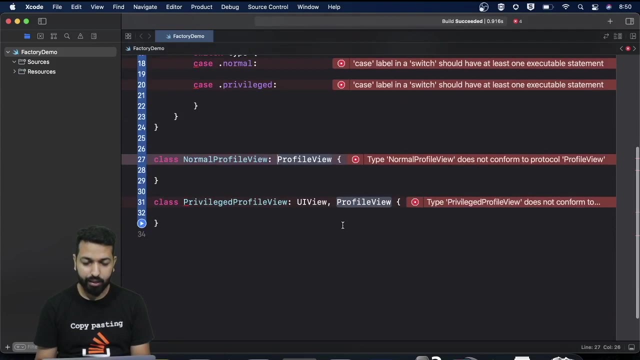 This will also be a UI view and profile view And if you want to impose this inheritance of the UI view, you can do that through the protocol. So if I write UI view here and then if I try removing it from here, I'll get an error saying that this normal profile view must inherit UI view. 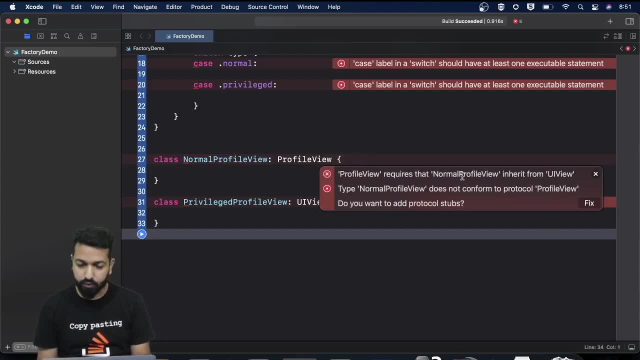 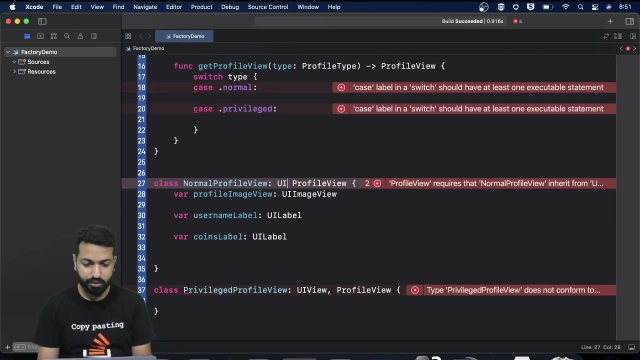 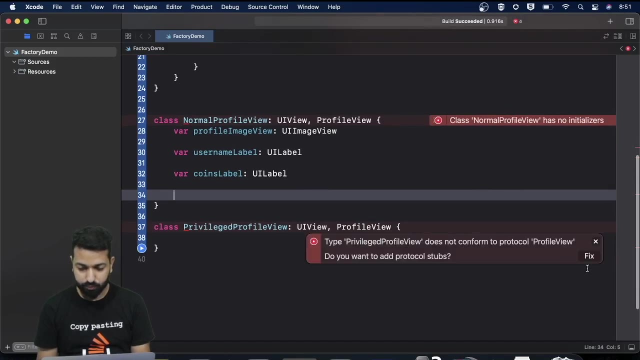 Let's see what it is saying. Profile view requires that normal profile view inherit from UI view. So let's fix it. Let's inherit from the UI view, and the inheritance should come before the conformance. Same should be done here. And then there's the initialization part of these views that I'm not covering here. 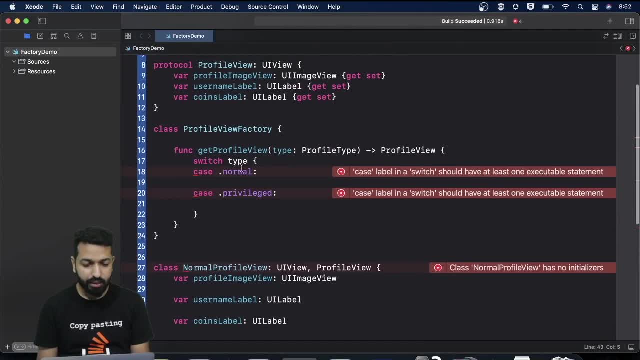 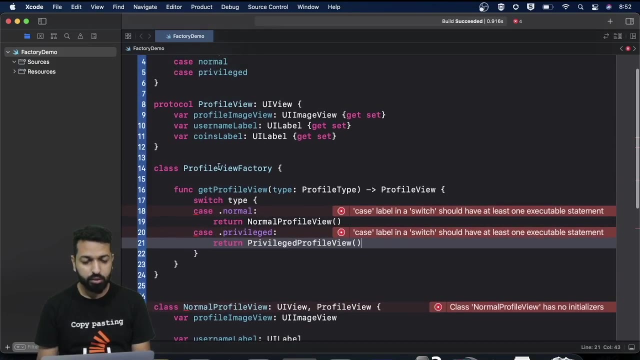 because this video Is not focusing on how to create the views, instead from these cases. Now we can return our different views that we are having. So we are having a normal profile view here and we have a privileged profile view here, So we can return it from here. 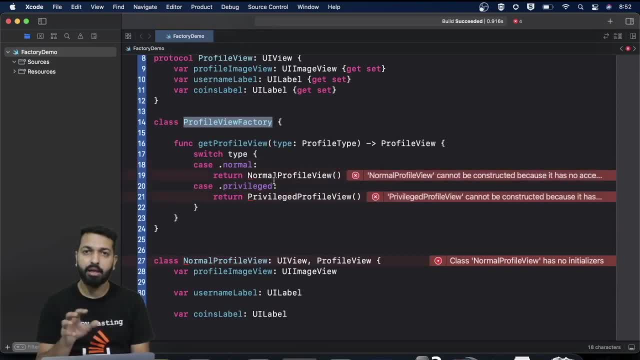 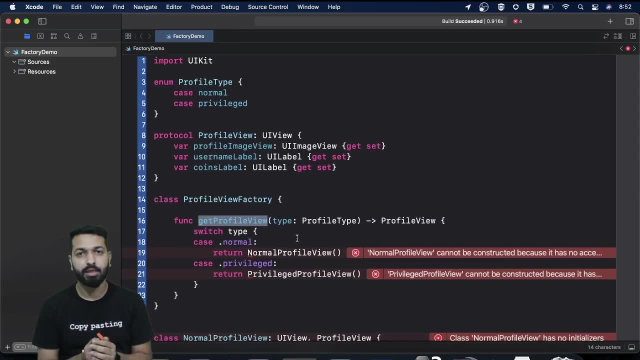 So basically, our profile view factory is creating our profile views and we are directly getting it by just calling this method: get profile view. Now there can be even more complexities. Now consider that Your company has got the projects from two different football clubs- let's say Barcelona and let's say Real Madrid- and you are asked to write a. 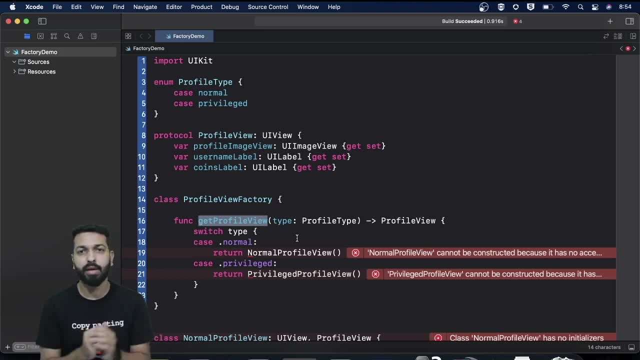 framework that should be responsible for creating the profile views for these two different applications, one for Barcelona and one for Real Madrid. Now, obviously, both the applications will have different theme And, considering this use case for those applications, that there will be a superstar user and there will be a normal user- 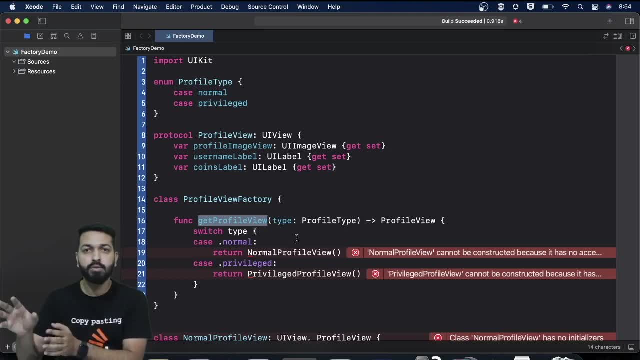 So basically, there will be a different superstar user, a different view for the user for Barcelona and the different view for the superstar user. So basically, each application has two views and in totality, you should have four views. Now how to deal with this scenario? 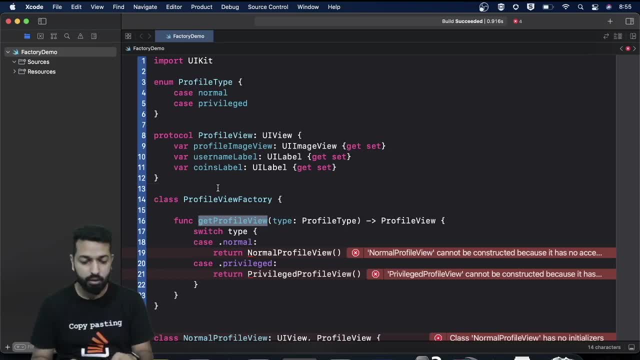 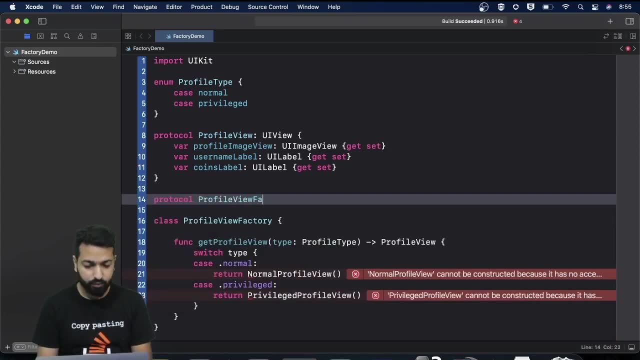 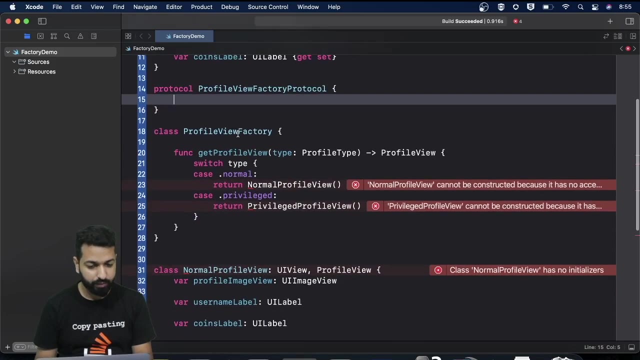 Now if you create one more protocol for that to which your factory confirms. So what I mean to say is that if you do something like this, protocol, profile, view, factory and, let's say, protocol- not the best way, but it's fine for now. 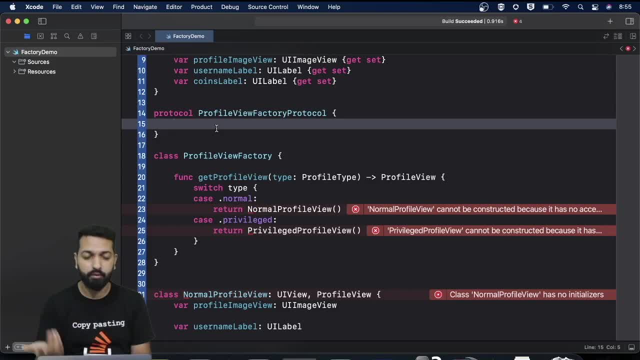 And in this protocol you define that your factory must have the method for get profile view. So if I go for fun, get profile view and you mention it here that it should receive a profile type, it should also receive the user object. let's say I'm not having user as of now. 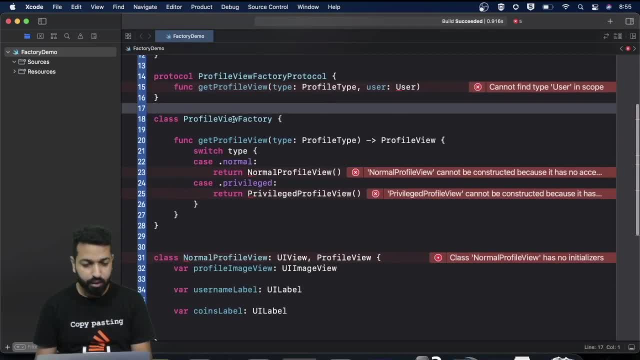 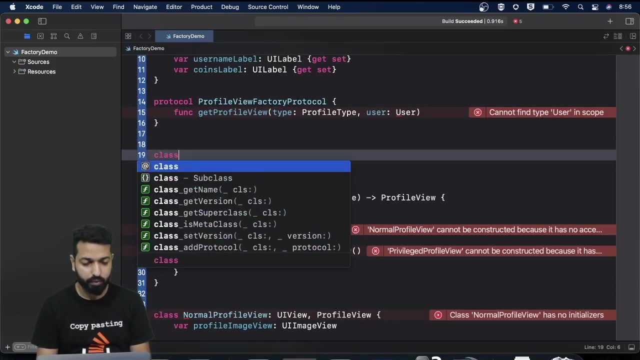 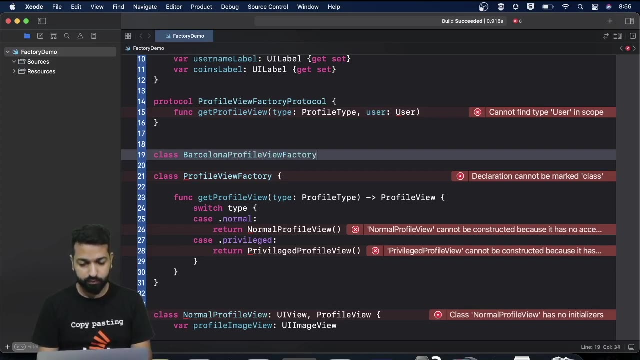 But yeah, that's fine for the example, just an example, And then all of your profile, your factory should confirm to this particular protocol. So if I go for, let's say, Barcelona profile view factory, which should confirm to profile view factory protocol. 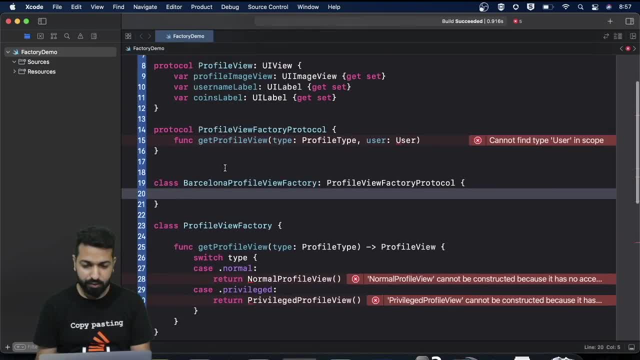 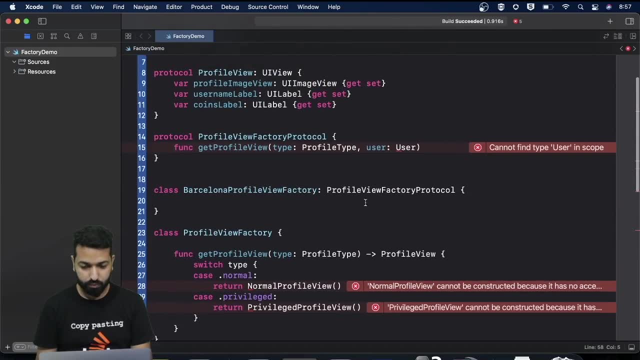 And then I have to write this method, that is, get profile view. So let's first fix this error. that is for users, So let's say struct user. Now I need to write implementation for this method, so let's go for it. 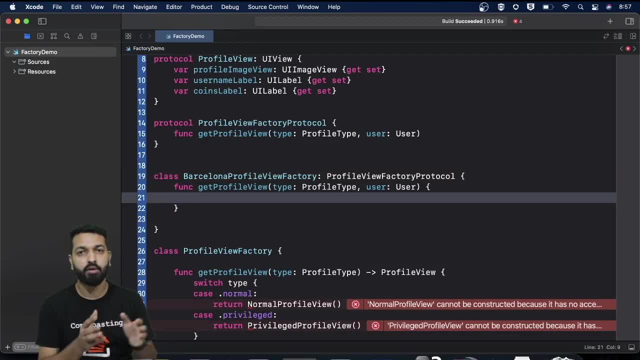 And inside that I can have implementation, depending on the Barcelona. Similarly, I can have a factory for Real Madrid. So this is where protocol comes to rescue. So the idea is that you should have the factories which will be responsible for returning the objects to you. 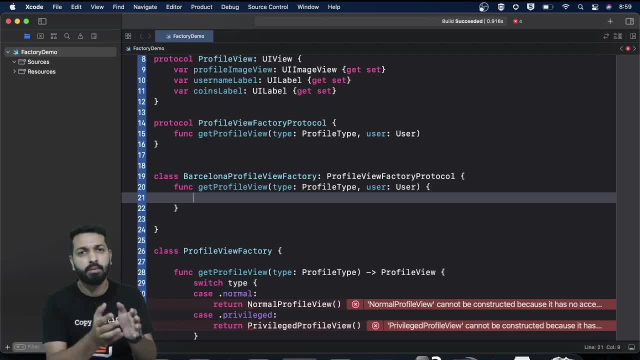 You can set up protocols, you can set up interfaces for imposing the guidelines or minimum set of requirements, and then factories can confirm to that particular protocol, Or I should say that those factories will be returning the object which are confirming to that particular protocol.